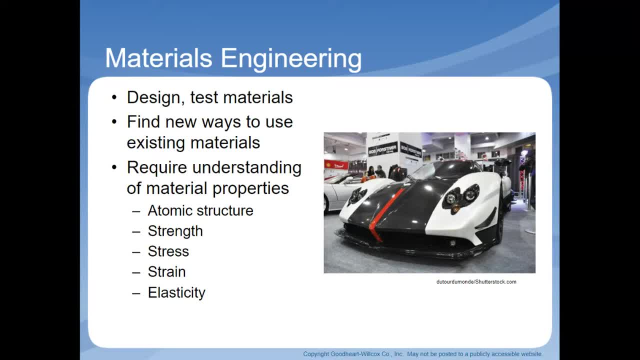 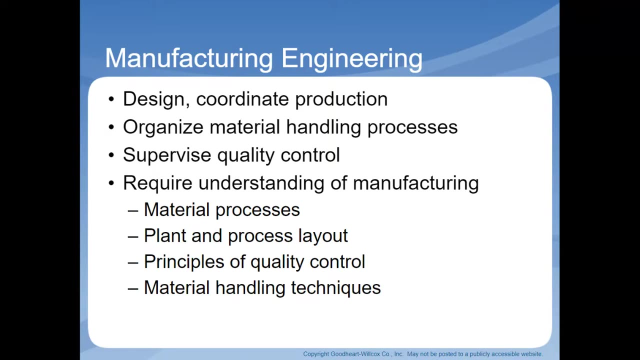 engineer that designs engines for cars. They would design the exterior of the vehicle, the materials that it's built out of: plastics, fiberglass or metal. Manufacturing engineering: They design and coordinate production, organize material handling processes. They supervise quality control. They require. 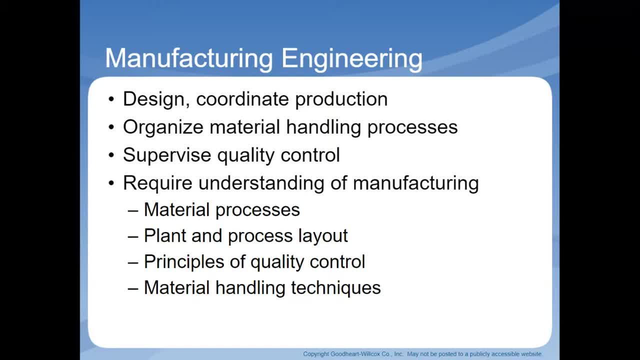 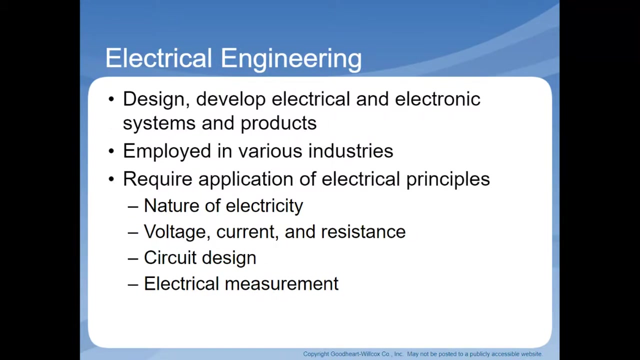 an understanding of manufacturing material processes, plant and process layout, principles of quality control and material handling techniques. If, looking at the prior examples of automotive, a manufacturing engineer would design the plant where the cars or engines are built, Electrical engineering: They design, develop electrical and electronic. 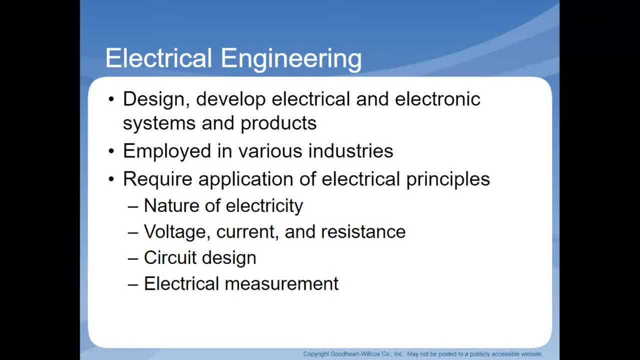 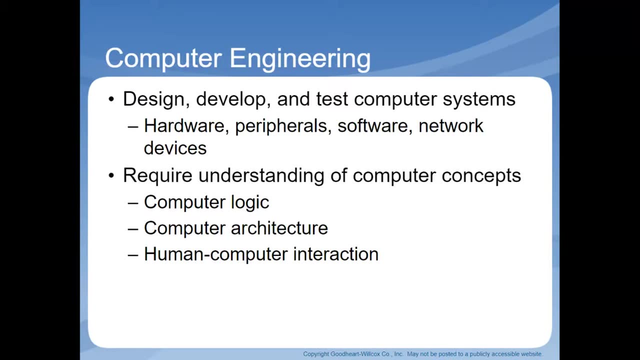 systems or products Employed in various industries. they require application of electrical principles such as nature of electricity, voltage, current and power. Electrical engineers would design and coordinate production, organize and voltage, current and resistance, circuit design and electrical measurement. 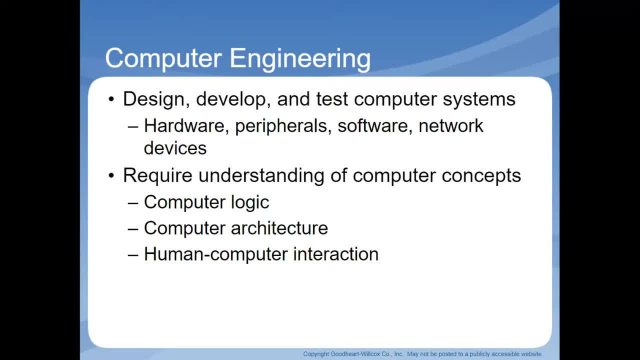 Computers engineers design, develop and test computer systems, hardware, peripherals, software and network devices. They require an understanding of computer components and concepts such as computer logic, computer architecture and human to computer interaction. The civil engineer is the design and construct public works projects. 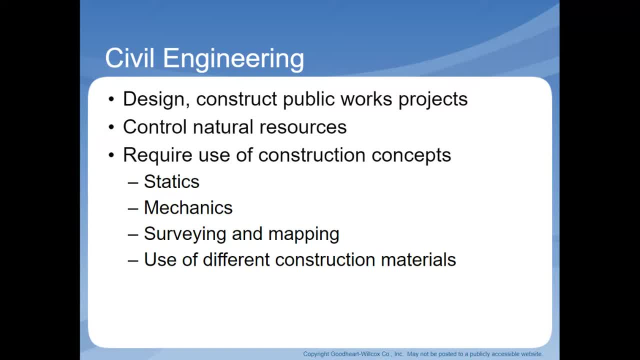 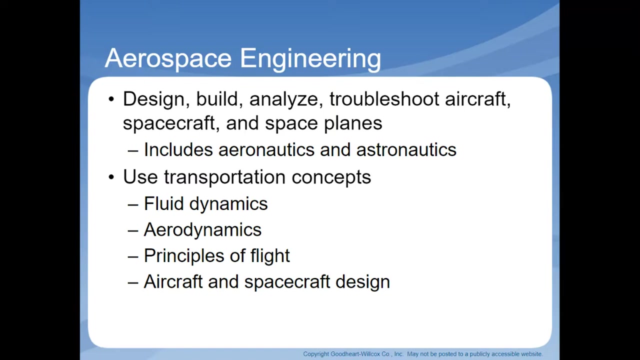 They control natural resources and require use of construction concepts such as statistics, mechanics, surveying and mapping, and use of different construction materials. An example of a project that a civil engineer may work on would be a building or bridge. Aerospace engineering designs, builds, analyzes and troubleshoots. 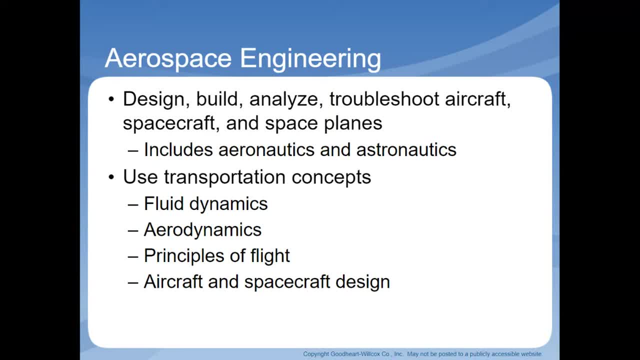 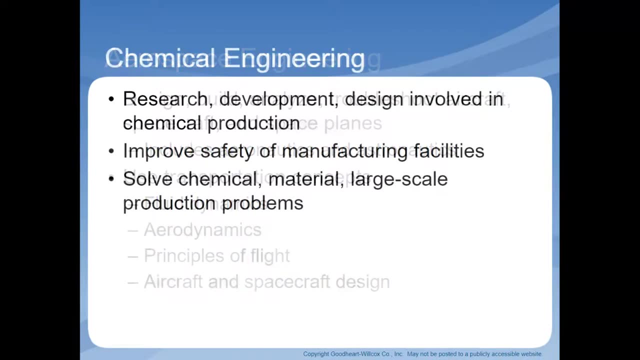 aircraft, spacecraft and space planes. includes aeronautics and astronautics. Use transportation concepts such as fluid dynamics, aerodynamics, principles of flight, aircraft and spacecraft. design: The chemical engineer: they research, develop, design involved in chemical production.